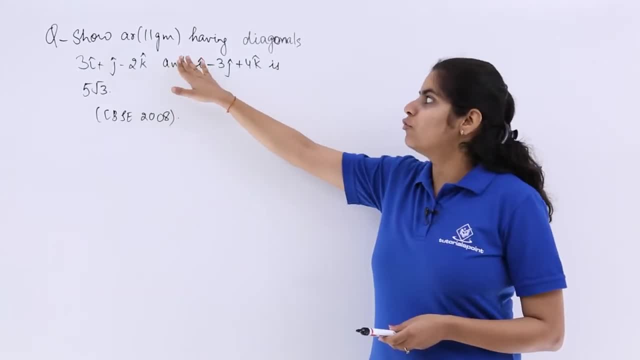 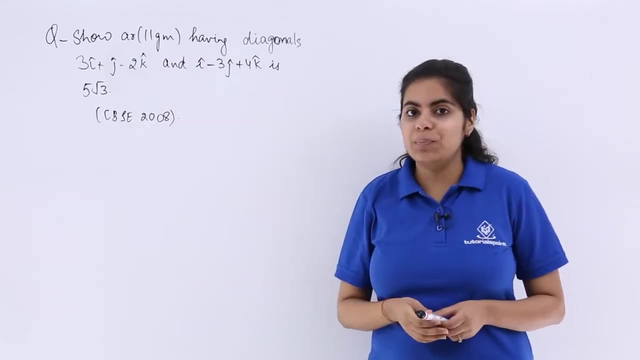 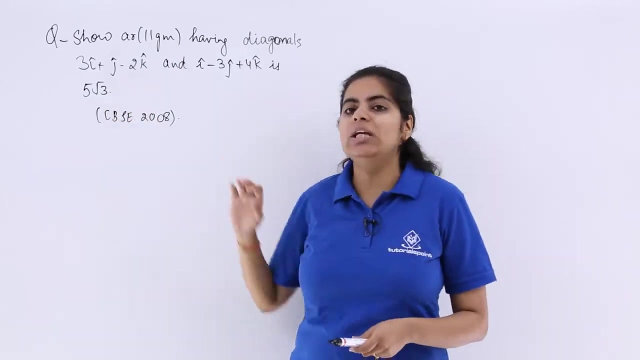 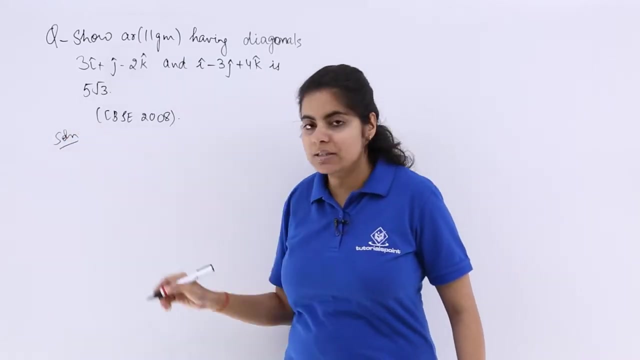 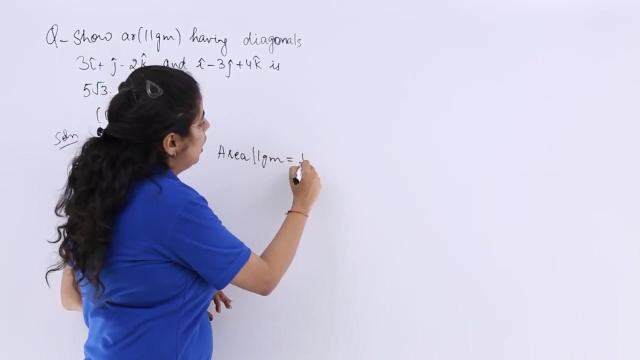 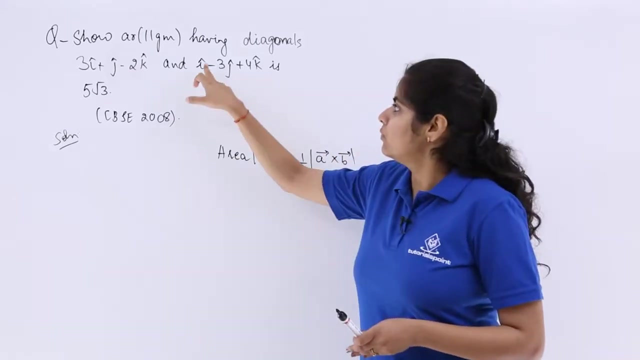 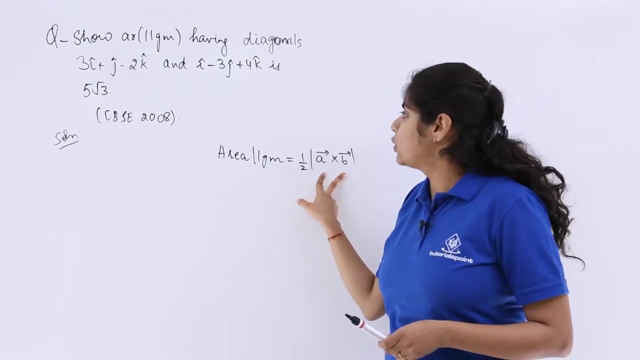 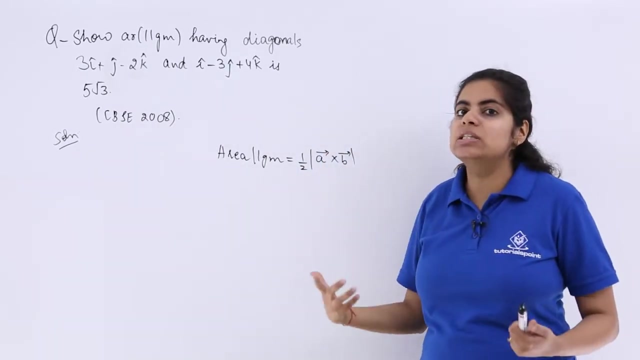 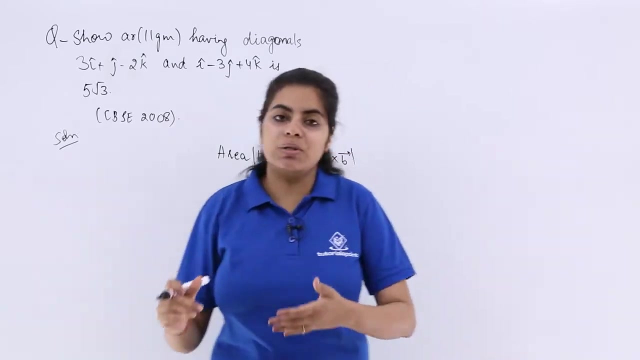 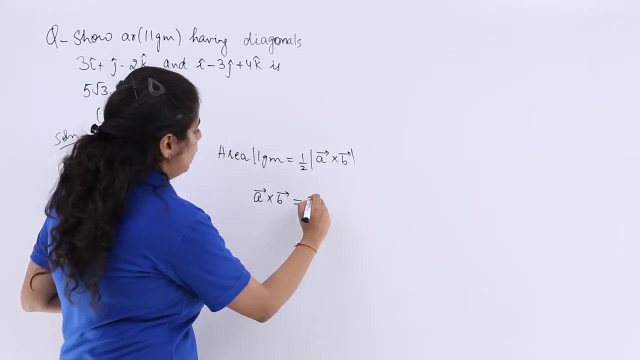 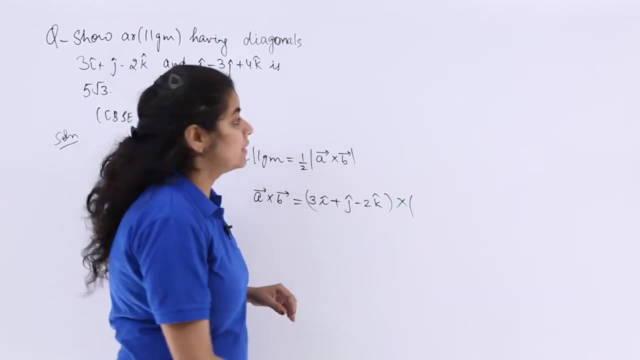 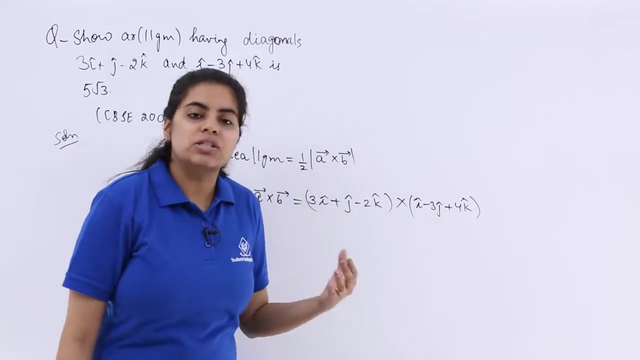 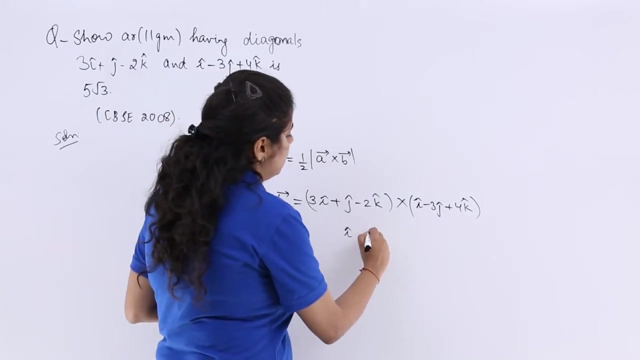 The question says, so the area of parallelogram, I have written in short for you, having the diagonal 3ic plus jcap minus 2kcap and icap minus 3jcap plus 4kcap is 5 root 3. So you have to find out the area and that area should be equal to 5 root 3 square units. So what is the formula of the area of parallelogram when we talk about vectors? I can compute the area of parallelogram by the formula of half modulus of a cross b where a and b individually are the diagonals. So the first diagonal is given to you and the second diagonal is given to you. So if you put the a cross b, this is a, this is b, if you take the vector product and then put here, then definitely this will give you an answer. So first of all, before finding out the area of parallelogram, you have to compute the area of parallelogram and then after finding the magnitude, you have to find a cross b. So let's find out a cross b. So what is a cross b like? I have to basically find the cross product of 3icap plus jcap minus 2kcap, the cross product of this first vector with icap minus 3jcap plus 4kcap. So this has to be done by the determinants method. That is the short trick. So since it is the first question, let me explain you from the very basic. So what you will do is you will write individually the unit vectors which are participating, that means icap, 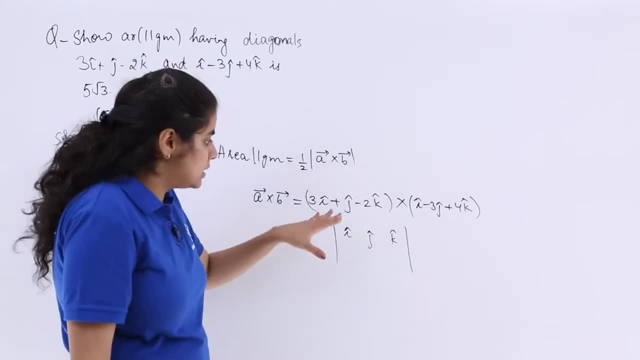 jcap, kcap and in the order, the first thing, the second thing, please mention which order you are talking about. 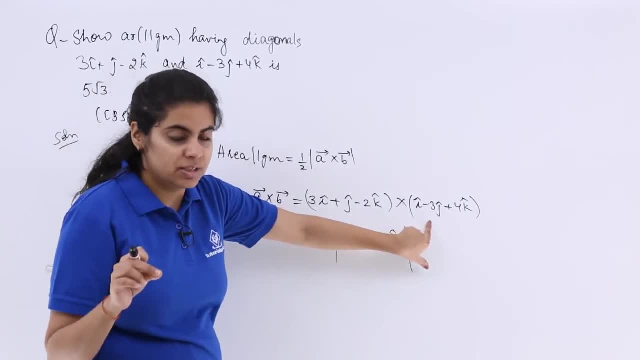 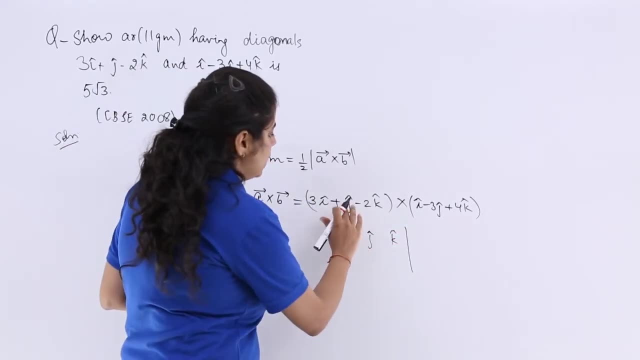 So if it is a cross b, the first vector is a, the second vector is b. If it is b cross a, the first vector is b, the second vector is a. Now this has the coefficient 3, j has the coefficient 1. 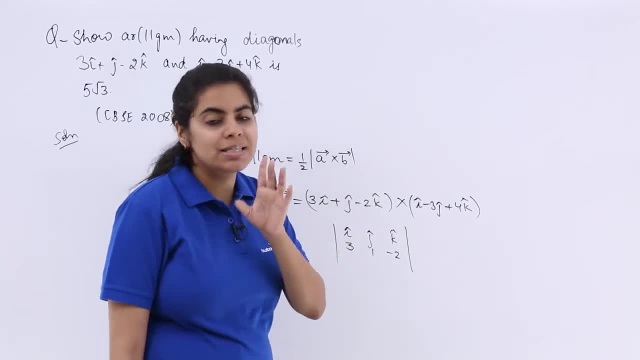 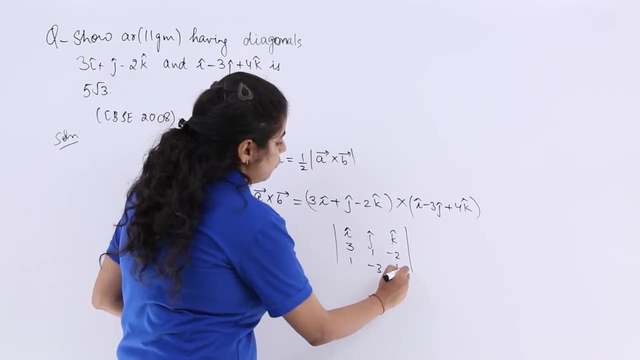 K has the coefficient-2 that means you have to take care of the sign as well. Talking about the second vector coefficient 1-3, 4 so 1-3, 4 this has to be done.